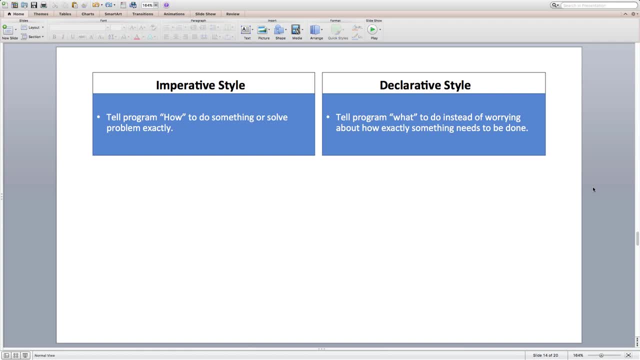 In fact, we don't need to repeatedly look into our inbox for newer emails. That's very comfortable, right? And that's where the declarative style beats imperative style: Simplicity and elegance. In imperative style, we tell how exactly we want to achieve the result, But in declarative 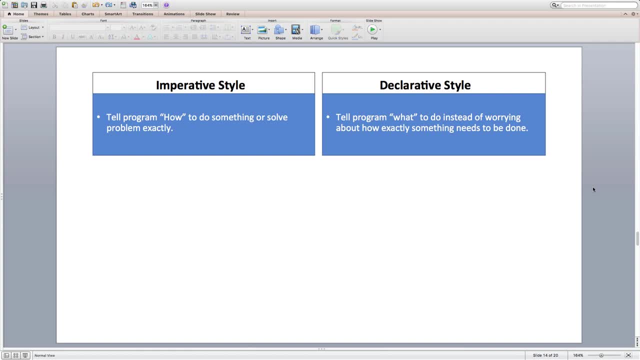 style. we actually say what result we want to get, Or what exactly we want to do, And the abstraction- like Gmail app in this case- just knows how to do it. Let's just look at one more real world analogy, Then we will jump right over to how imperative 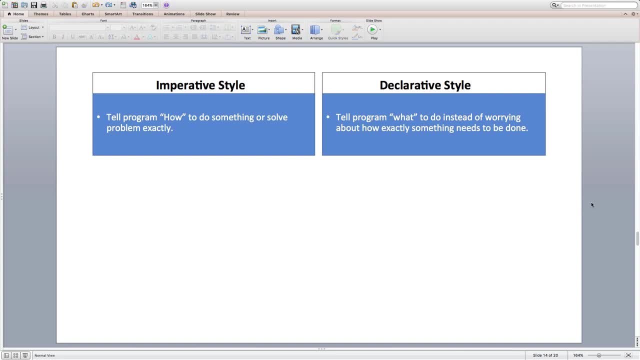 and declarative programming looks like in code. Let's say I need a desktop that should have the specifications of 8GB RAM, 256GB SSD hard drive and Intel i7 quad core processor. There are two ways that I can get a computer of. 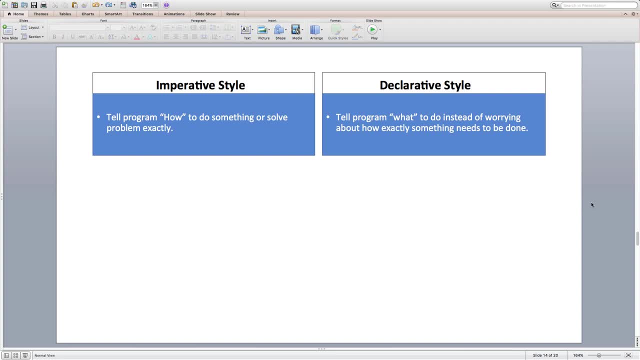 my spec. First way would be an imperative way Where I can order individual parts from Amazon, Like buy a 8GB RAM, buy a 256GB SSD hard drive, a CPU cabinet, an Intel i7 quad core processor and a motherboard- All parts separately. Once I have all the parts, I will 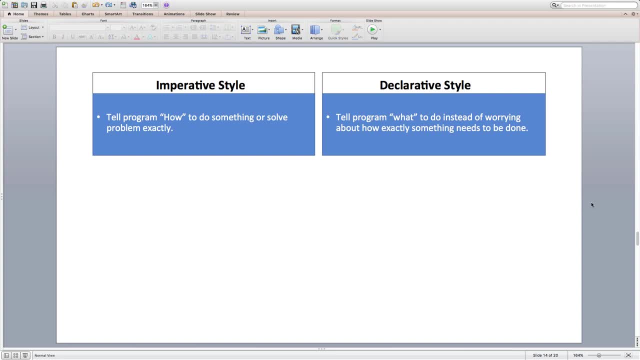 assemble these parts together to create my desktop. That's very much imperative style. I am the one who is deciding on how to create a desktop, given. I know how to do that. So here we are telling on how to do something. Same thing I can do in declarative way by: 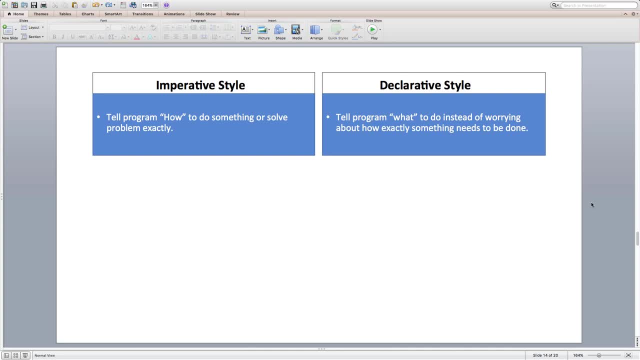 just searching for desktops on Amazon and providing filters according to my requirement, And Amazon just knows what desktops are available with my matched specs and displays them to me In declarative way. I am just telling what I want And in this case, Amazon just knows. 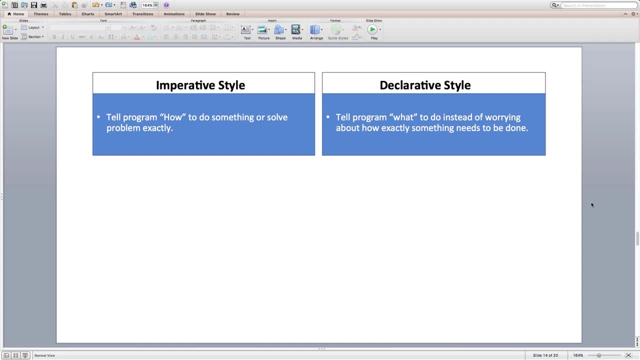 how to do things for me. Now you might notice that imperative style provides much more flexibility. I can take RAM from X company, hard drive from Y company, cabinet from Z company, and so on, And I can assemble these different parts as I would like to. 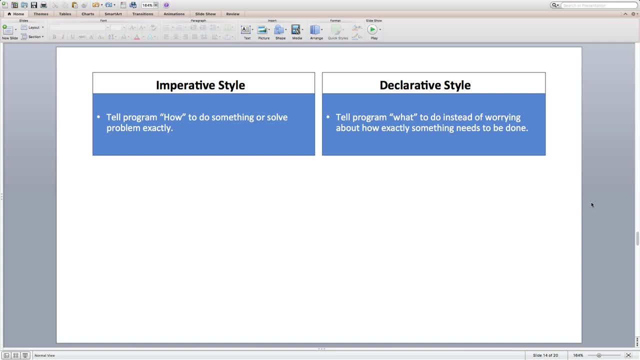 In declarative way. we have limited choices. We would have to rely on desktops available on Amazon or any other e-commerce store that match our specs, Even though imperative way provides us flexibility. most of the time, I might not want flexibility. Actually, I don't need to know how to assemble a desktop in order to use it, I just need. 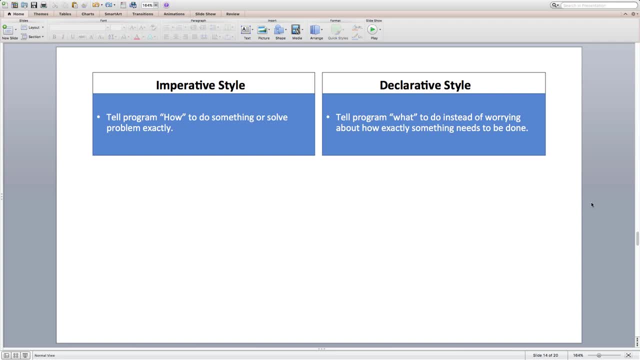 to know how to do something. I don't have to know how to do something, but I just want to say what would I want to have So, imperative way provides us the flexibility but brings in some complexity, Whereas declarative style provides us simplicity and hides complexity, But in some cases it may not solve what exactly. 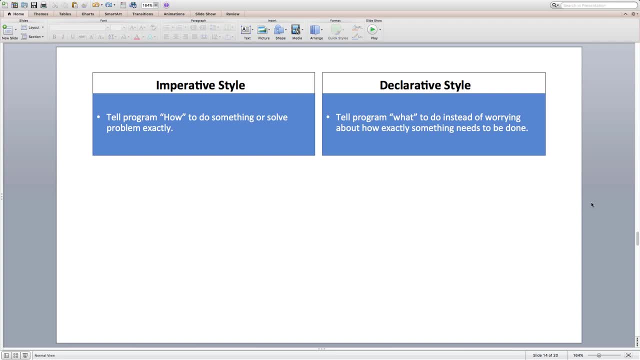 we want it to. Both the approaches are important, but always prefer declarative way if you don't need any flexibility. Declarative style is just telling what we want to achieve or do something, but not how to achieve, Whereas imperative style tells how to do something. 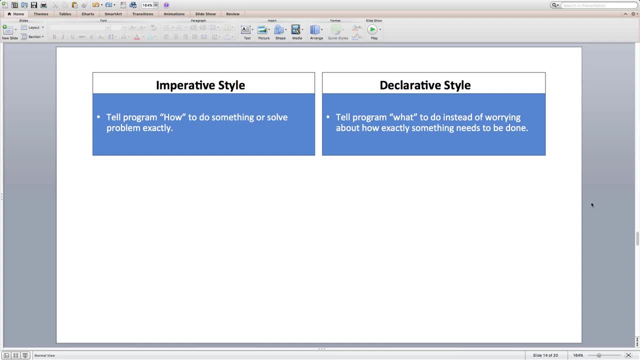 So I don't have to know how to do something, But I just want to say what would I want to have, how we want to achieve or do something. I hope it makes a little bit of sense now. Alright, let's now talk about. 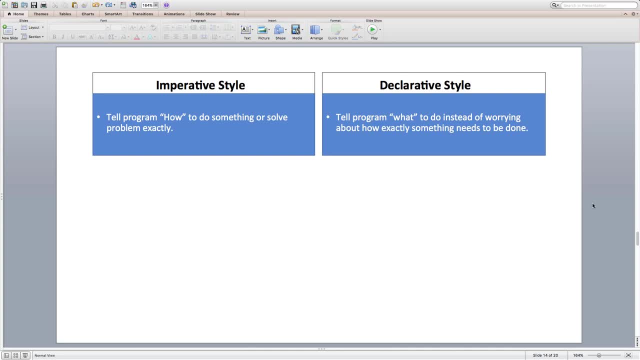 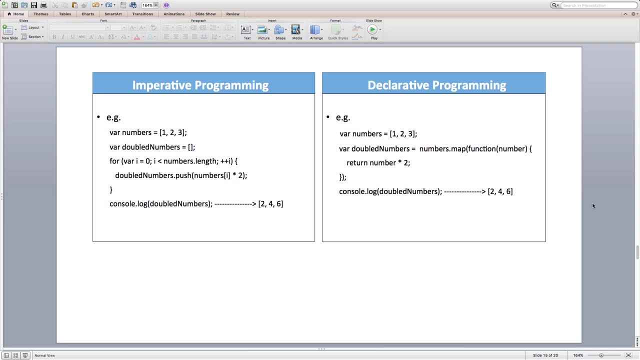 imperative and declarative programming. Let's look at a very trivial problem now, Given an array of numbers, we need to create another array that has numbers twice of the given array, keeping the order of elements intact. Let's say I have numbers array containing one, two, three. 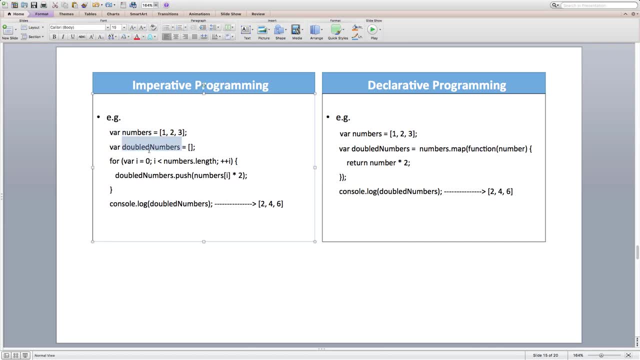 And I want the resultant array, double numbers, to contain twice of each element in my numbers array, So effectively. I want it to have two, four, six. Okay, we can solve this problem in two ways. One way is imperative and the other way is declarative way. 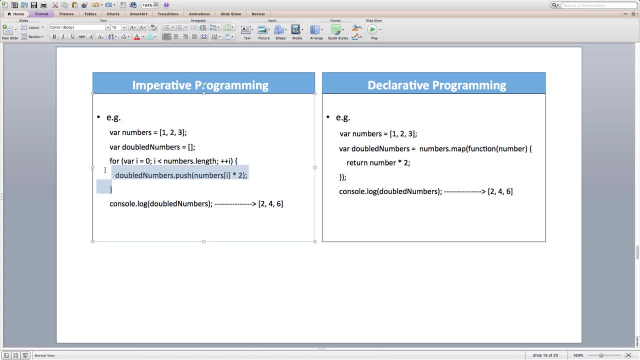 Let's see how it can be done imperatively. This is the crunch of logic here. Here we are saying that I want you to create a variable i and initialize it with zero and check if i has crossed the total array length. If not, then I want you to run the body. 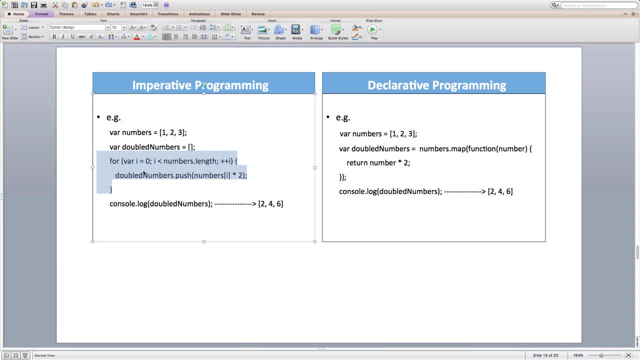 Inside the loop, multiply numbers of i by two and push it into an array double numbers, Then I want you to increment i and run the loop body as long as all the numbers inside my numbers array are processed or covered By doing this, our double numbers array. 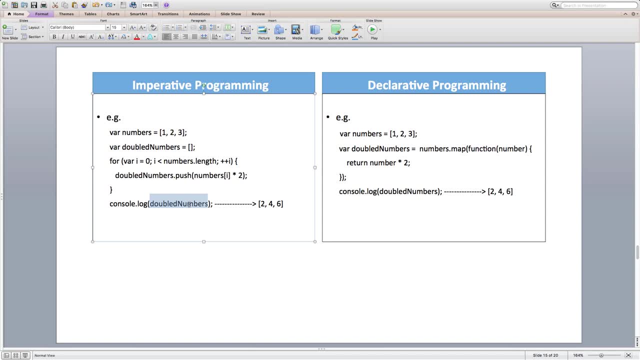 will be filled with two, four, six. This is the imperative way of doing it. Let's see how we can do the same in declarative way. Again, this is the crunch of logic over here. By invoking dot map here we are telling it. 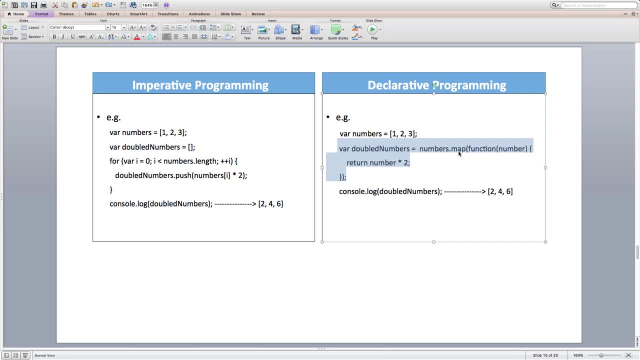 can you just iterate over each item in my numbers array and trigger my callback function with each item one by one, And store the return value into a new array before assigning the final computed array to my double numbers over here? With this again we get our double numbers array. 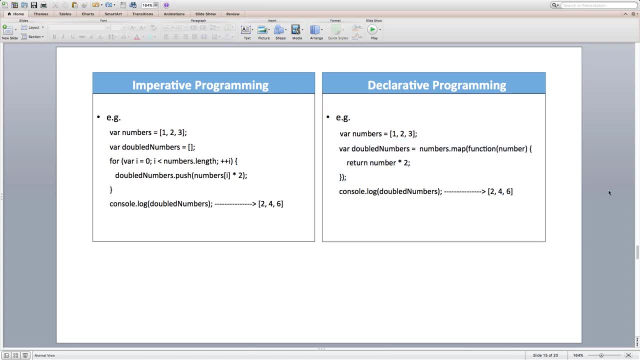 filled with two, four, six. So we'll get the same result using two different methodologies. If you observe, in imperative programming we are telling each and every step to the program, like how we want to iterate over an array that is increment by one. 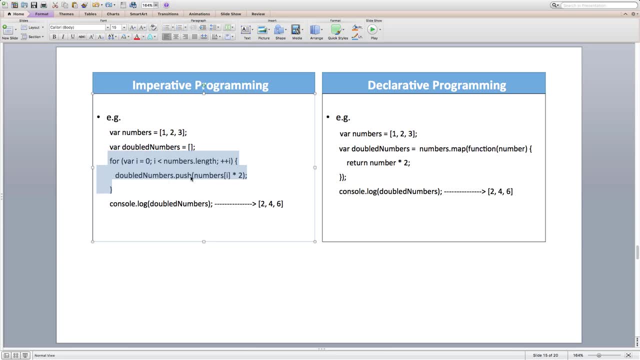 and how to push a computed value into a new array, that is, use dot, push over our resultant array like this: This is in fact saying how to perform each and every step to store the computed values in our resultant array, Whereas in declarative programming, 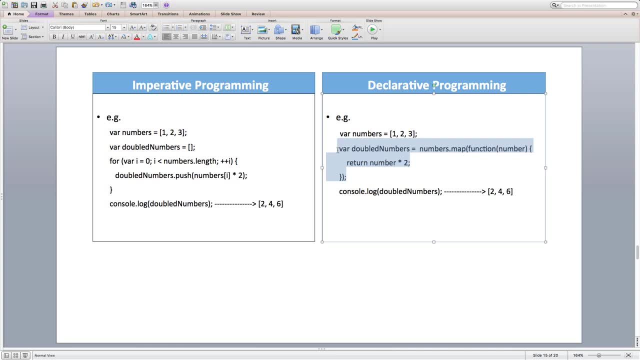 we only tell what is our main objective, that is just to double the numbers. So we tell the computer only the minimal thing, which is for each number in our numbers array. we return a new value that is twice of the existing value through the callback, and that's it. 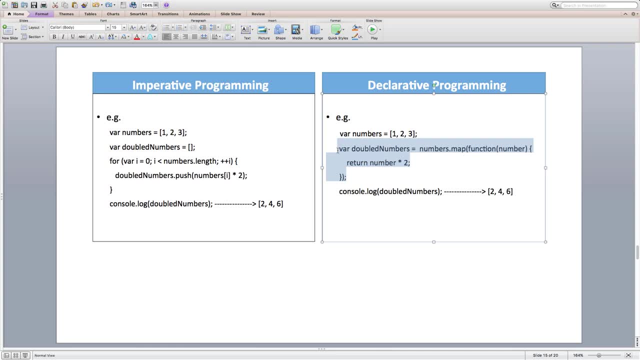 We leave the rest to our map function. It knows how to iterate over an array. It also knows how to push an item into the new array And finally it returns a computed array. We are just telling our computer what is our main objective here. 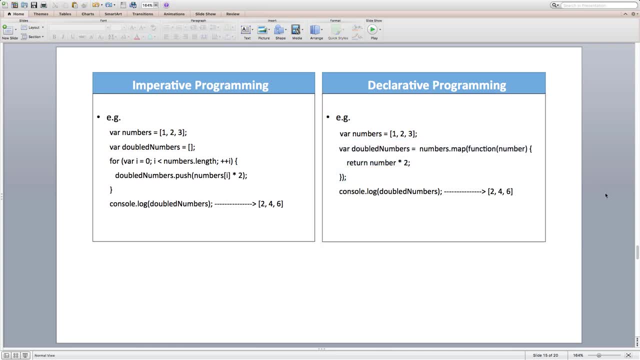 and what should be the end result. Iterating over all the items of an array and constructing a new array is one of the most common patterns that we'll see, especially in front-end development. So, instead of us iterating over an array, we converted this pattern to a higher level API. 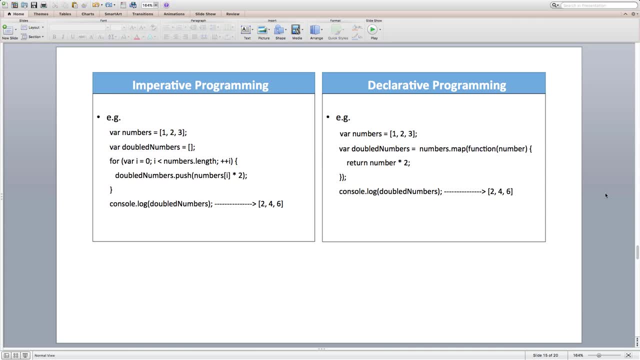 or abstraction, called map For starters. map function is a kind of abstraction that knows how to iterate over an array and push items into the new array before returning the computed array From our side. we just need to know how to tell that abstraction. 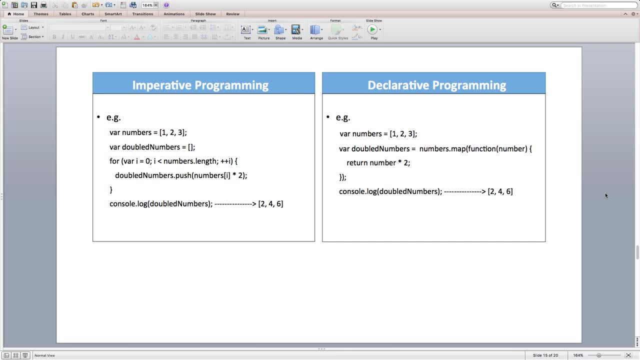 what particularly needs to be pushed into the new array and map will take care of everything else. That's why we created these utility functions and libraries like underscore, low dash, et cetera, Instead of doing the same thing again and again. 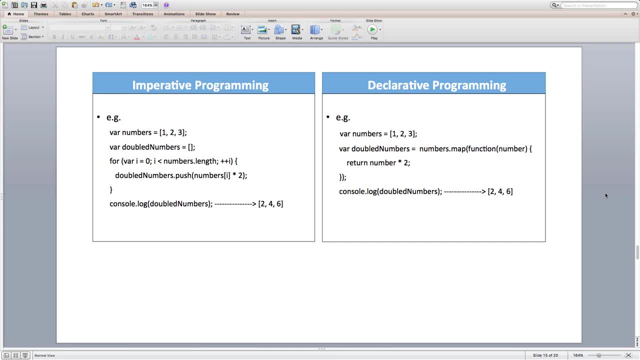 we use these patterns, functions and abstractions to help us do what we want to, rather than we worrying about how to do something With declarative programming. writing less code and logic is just a bonus, apart from better readability. One final thing here.